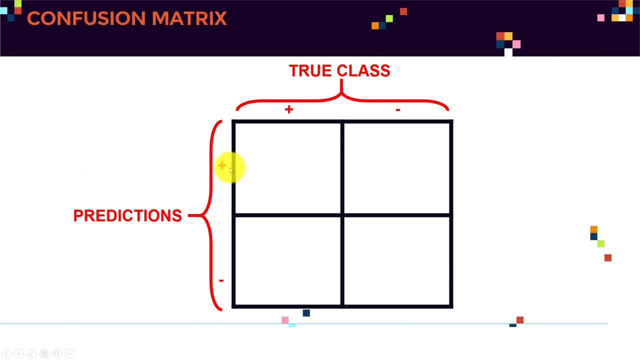 So for example, here the model might say positive or negative, which means two classes, either one or zero, and here my true class is either one or zero. So if my model predictions matches my true class, these are what we call true positives. 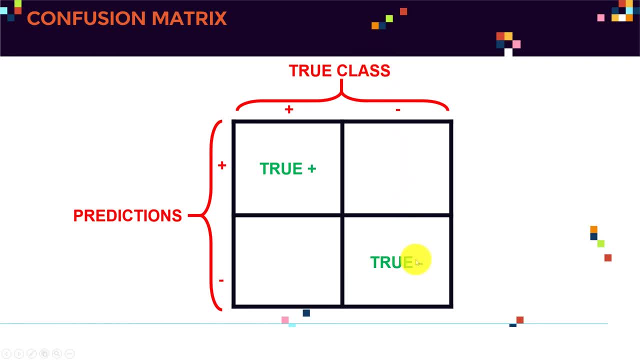 If my model predictions matches my true class, matches my true class. okay, if my model predicted, let's say, negative, for example, and my true class was actually negative, that's what we call true negatives. And then that's here. we mark them as green, because that's when everything is good, you know, when everyone is happy. 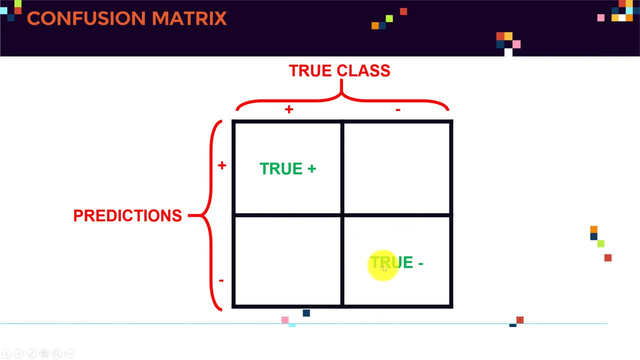 I hope my model will be able to get you know all the true positives and the true negatives. However, that's not what happened in reality. What happened in reality is sometimes the model messes up, which means the model might predict leeway. 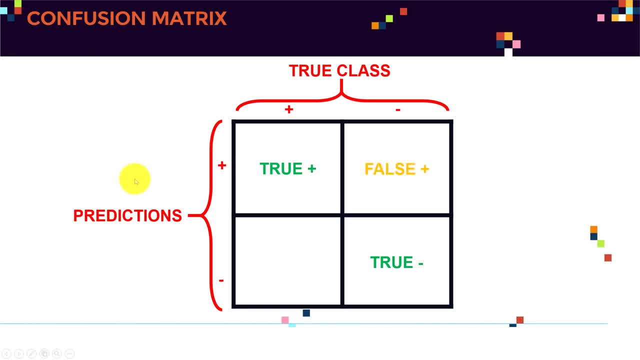 So it might give a positive Level 1.. So, for example, the model might say that the patient has, let's say, cancer, for example. So that's positive. However, in reality, the true class was actually negative. In reality, my patient was actually cancer free. 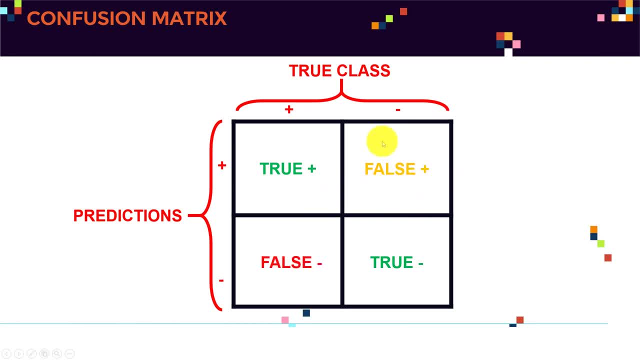 And that's what we call it false positives, And we call this type of errors Type 2 error. Okay, Which is, And we call this type of error Type 2 and Type 6 error type, and we call this type of error Type 2 error. 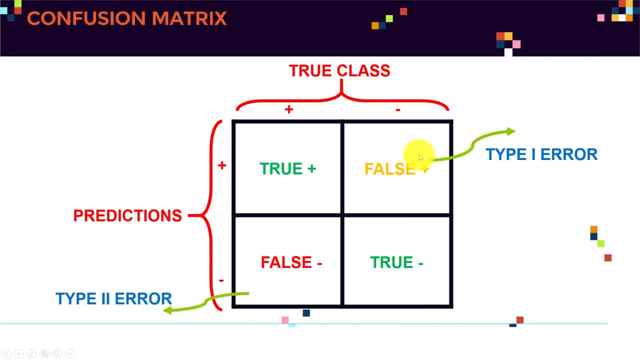 And we call this type of error Type 2 error, we call it type one error. okay, and we call it type one error because, yes, I understand it's still an error, yes, it's still a problem, but the patient it's still, is still fine. yes, we scared, you know, scared- him off by telling him that. 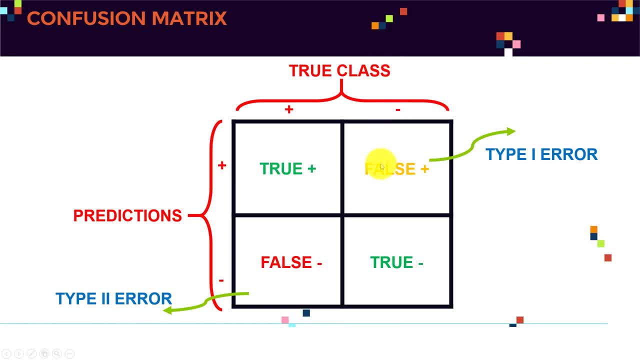 you have cancer, but in reality he was actually cancer-free, he was actually okay, he was actually fine. so that's what we call it. type one error, however. this is the problem. okay, that's the issue and that's why we mark this in red. that's when our prediction says we are negative, which means the model says: I do not. the 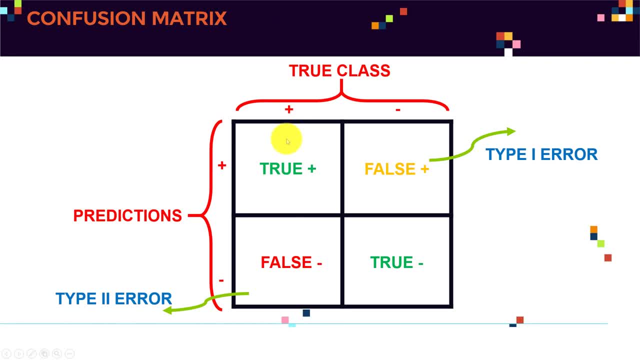 patient does not have cancer, that means negative. however, in reality, the patient did have cancer and that's a big issue and that's what we call a type two error and that's what we want to avoid at all cost. okay, because that means you know, if you don't treat him, him or her, then you know. 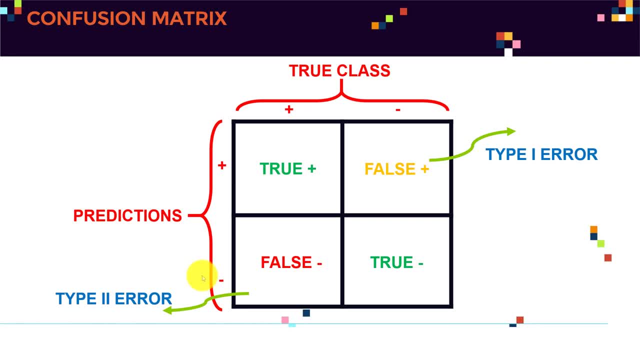 he the, the disease might grow, and then you know like that would be too late at some point. so you basically messed up big time here and that's why we call it type two error. all right, so let's take a look at again some of the definitions of, as I 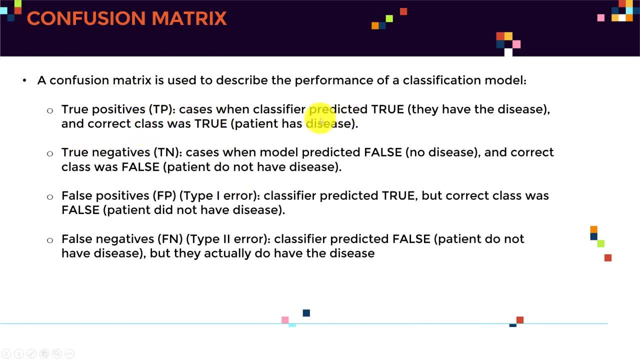 mentioned, we have two positives, which is cases when the classify classifier predicted true, which means that the patient had the cancer or have a disease, and the correct class was actually true, which means the patient in reality has a disease. so that's a true positive. true negatives are with the cases when the model predicted false, which means he. 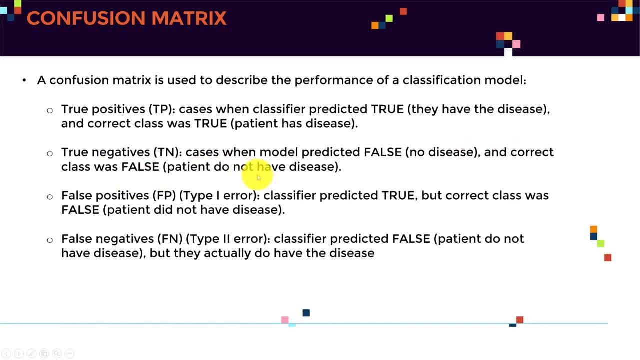 doesn't have a disease and in reality the patient was actually disease-free. it is an habit. it is an avid disease as well. these are ok. now to the problems. we have false positives, which is what we call it type 1 error. that's when the classifier predicted true, but the correct class was. 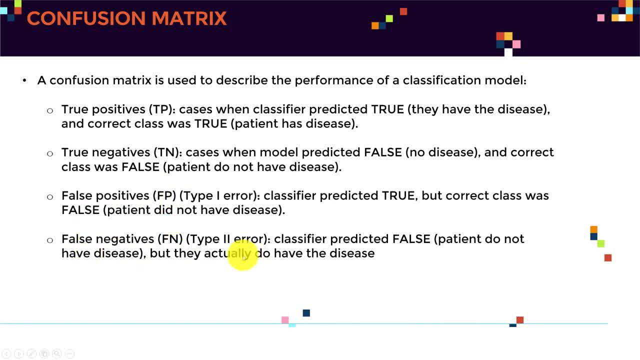 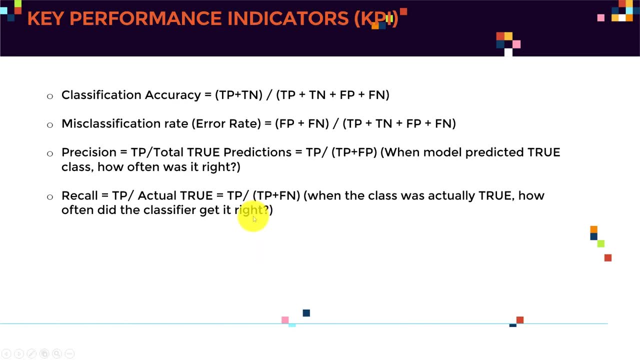 actually false and the false negatives are type 2 error. that's when the classifier predicted false, when we said that the patient does not have a disease, but they actually do have a disease in reality, and that's why we call this type two error. all right, so let's take a look at the key performance indicators, or 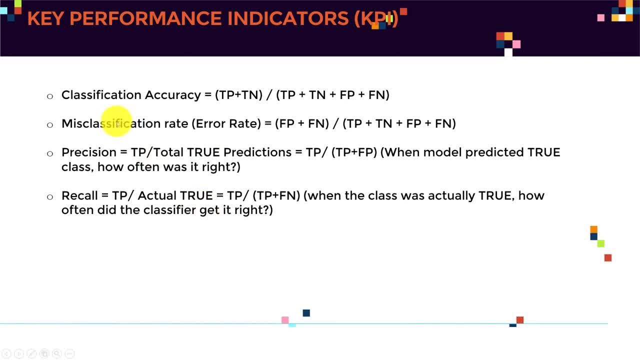 KPIs. what we do here is that we assess the performance of the classification strategy using these kind of. you know four main KPIs. first one is the classification accuracy. we simply sum up the two positive positives plus two negatives, we divide by the overall number of samples, which is two. 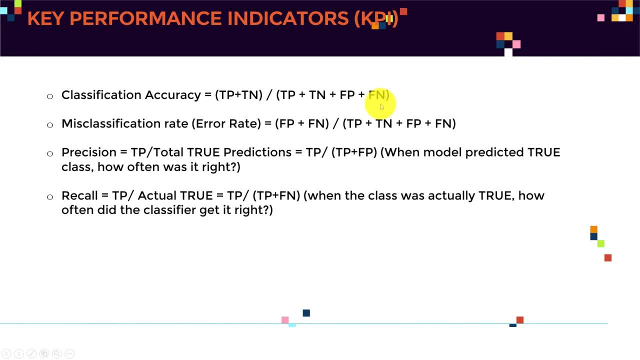 positives plus two, negatives plus false positive, positives plus false negatives. the other one is the misclassification rate or the error rate, which is simply, we sum up our how many times we messed up, which is false positives plus false negatives, and we divide by the total positives, true, positives plus two. 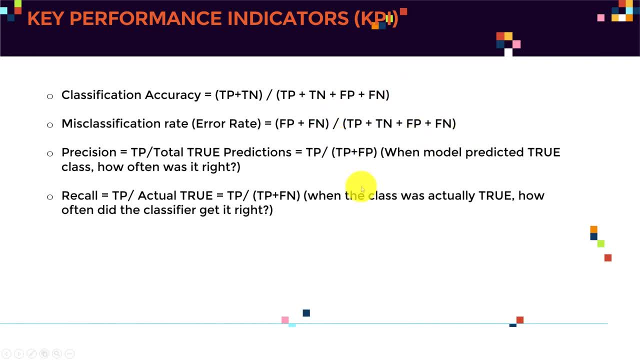 negatives plus false positive plus false negative, again the overall number of samples. and then these are the two important kind of, you know, different things that we can do to assess the performance of the classification strategy. definitions: when we assess the performance of a classification technique, and this is what we call it, precision and recall- precision is simply when the 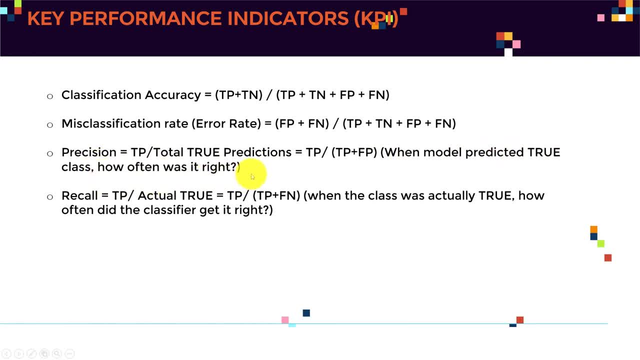 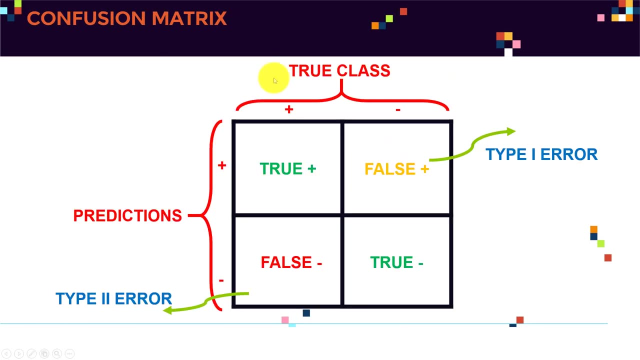 model predicted true. how often was it right? okay, so we take the two positives and we divide by the overall total two predictions. we simply divide two positives divided by two positives plus false positives. simply put here, when we take a look at this, we divide basically the true positives divided by true positives plus false positives. okay, 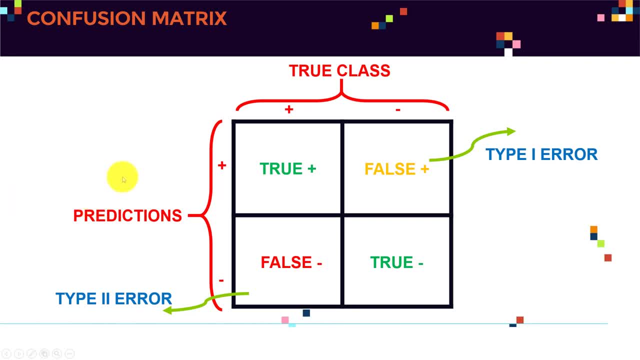 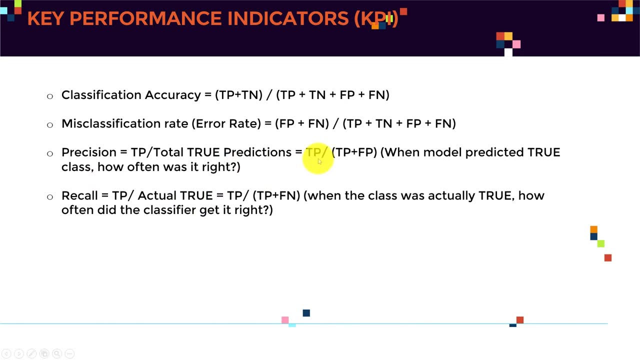 and that's what we call it precision. okay, which is simply when the model said that the patient has a disease, which means I'm here on this row, how many times I was right and how many times I messed up. basically, that's all what it is, and that's the first definition. the second definition is what we call as: 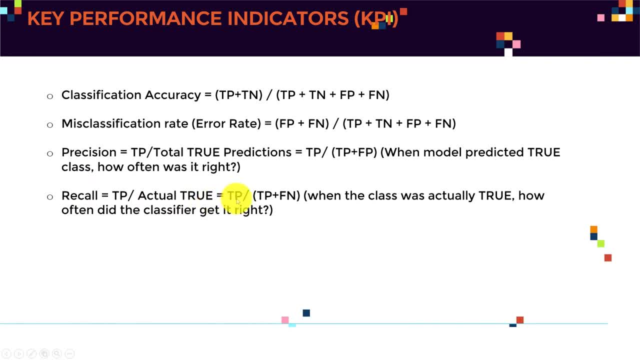 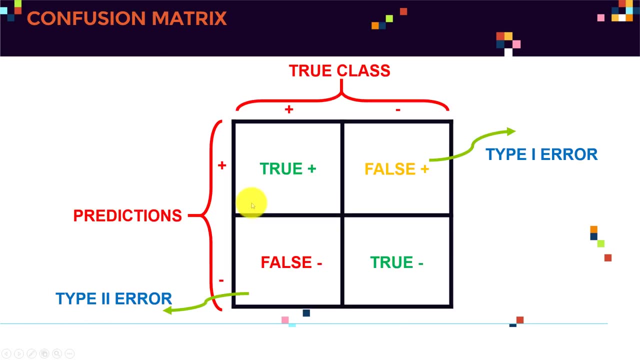 recall, which is simply we're going to divide the true positives, divided by true positives plus false negatives, which is, again to recall means: is that, when the class was actually true, how often did the classifier get it right? which means here, when the actual true, when, in reality, when the class was? 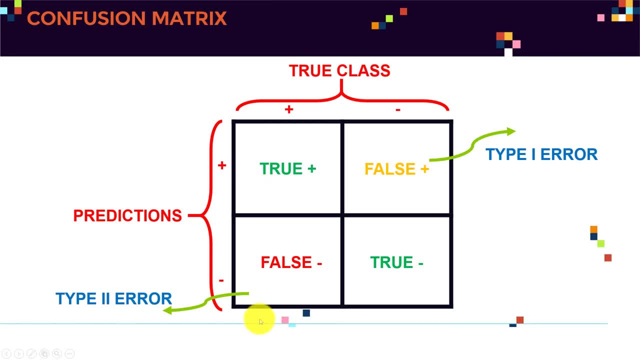 actually positive here in this column, how many times I got it right, which is mean how many times I have been able to detect these positive cases. okay, if you guys are confused, I know it's might sound a little bit confusing, so let's take a look at a practical example. let's assume 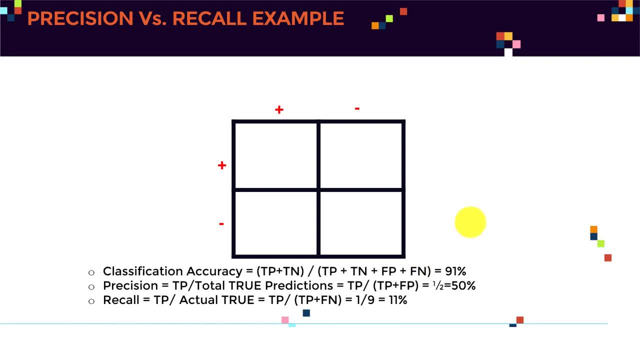 that I have hundred patients, okay, and out of these patients- actually I think I have here this numbers, so let's assume that, again, I have hundred patients, okay, and let's assume that I have, out of these hundred patients I have, 91 of them are cancer-free, so they are healthy patients, and I have nine patients who 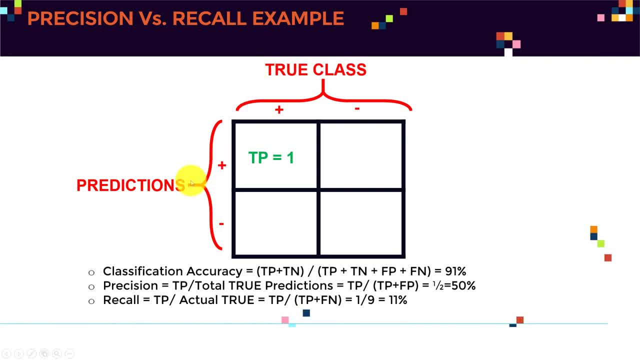 have cancer. okay, and let's assume that I train my classifier and I came up with these values. so now I have the classifier has been able to classify true positives equals to one. the classifier got true negatives equal 90, so he got 90 samples as true negatives and then the 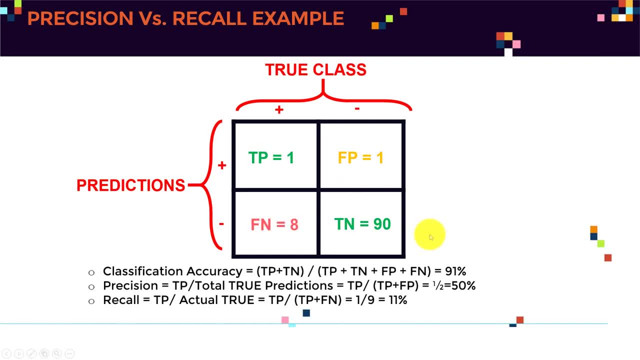 classifier got a false positive equals to one, and the classifier got false negatives equals to eight. okay, so if I give you this confusion matrix, could you please assess the performance of this? you know like artificial neural network or a classifier model, objectively? so first we say: you know. 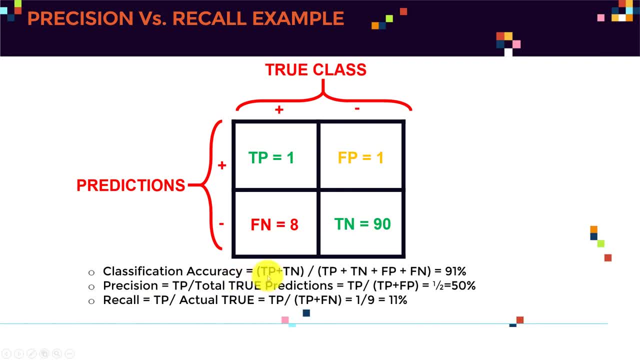 what. I will go and calculate the classification accuracy. I'm gonna sum up my true positives plus true negatives, which is simply 90, plus 1, which is 91, and I'm going to divide by the overall number of samples, which is simply a hundred, so I will come up with 91%. okay, so if you take a look at it, you will say: 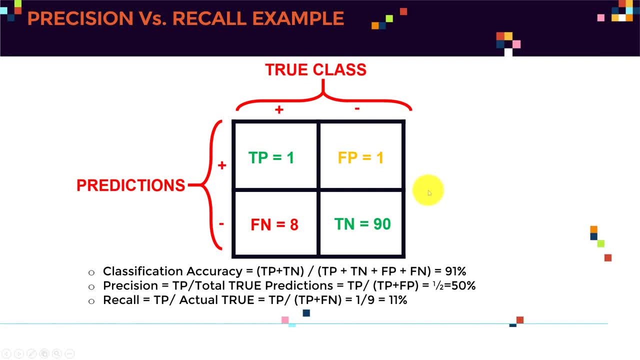 you know what this network is actually going doing. amazing: it got 91 percent accuracy. everything looks great. however, this network, in reality it's actually garbage. it's actually useless. let's see why is it useless. so, if we try to calculate the precision, we'll find that if we sum up true positives divided by 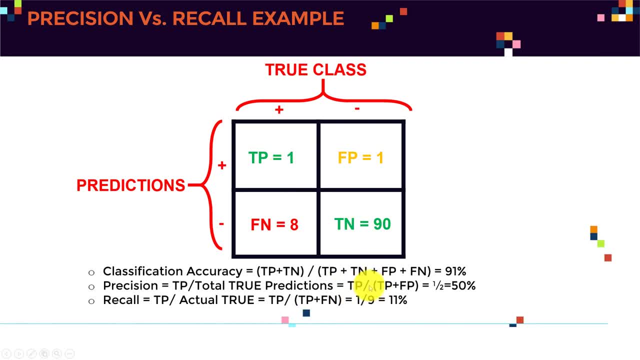 the total true predictions, I will come up with 1 divided by true positives plus false positives, which is half, which is 2. so I'm gonna get 1 divided by 2, so I will get 50%, which means the model is actually 50% kind of precise when it comes to making predictions- again, kinda useless. 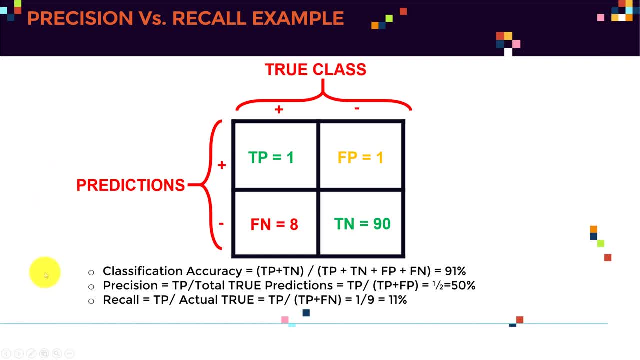 and if we take a look at the recall, which is again, out of these nine cancer patients, how many of them I have been able to detect? that's the exact answer. so, as you guys can see here, basically the network has been able to only detect one cancer patient. so it's 1 divided by 1 plus 8, so it's 1 divided by 9. 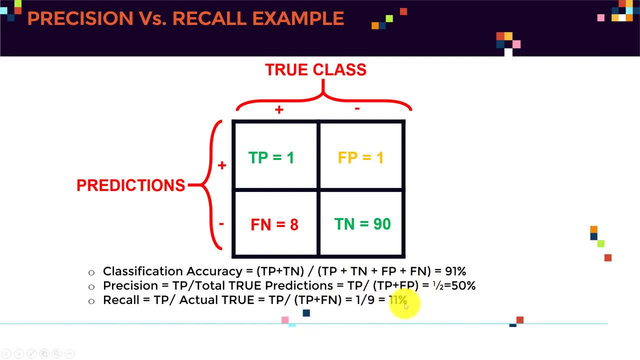 that's only 11 percent, which is horrible. okay, and basically, when we have an unbalanced data set, like in this case, when we have, let's say, 100 patients, 91 of them are healthy and 9 percent or 9 of them have cancer, that means it's an. 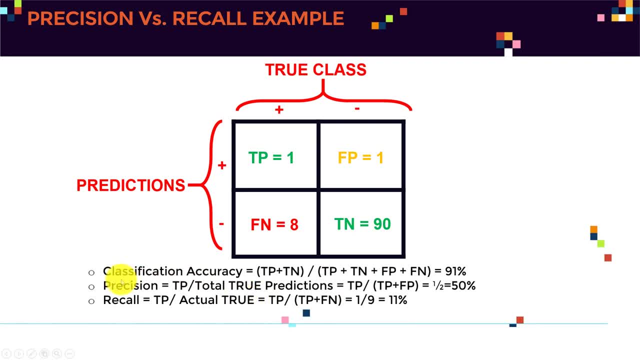 unbalanced data set. so now we need to actually take a look at the precision and recall to fully understand what's the performance of my classifier in this case and again, you will find that this network again is totally useless and because out of these nine cancer patients I've only got one cancer.